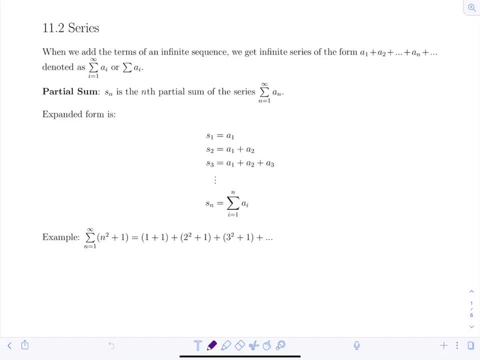 blah, blah, blah, up to an, which is the general term, and this could be denoted using sigma notation as the sum i equals 1 to infinity of a sub i, or just as the sum a sub i Now a partial sum s sub n is the nth partial sum of the infinite series from n equals 1 to infinity of a sub n. So to 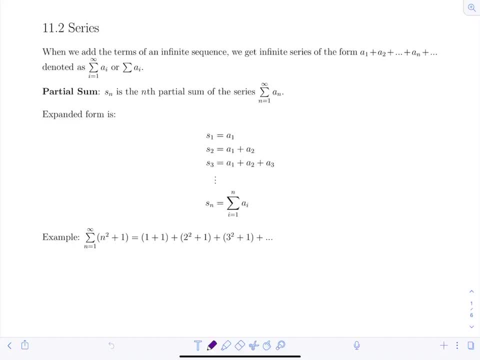 get an idea for what this partial sum is, let's look at it in its expanded form. So s1- the first partial sum, would just consist of the first term of the sequence a1. that's it. S2: the second partial sum is the sum of the first two terms. 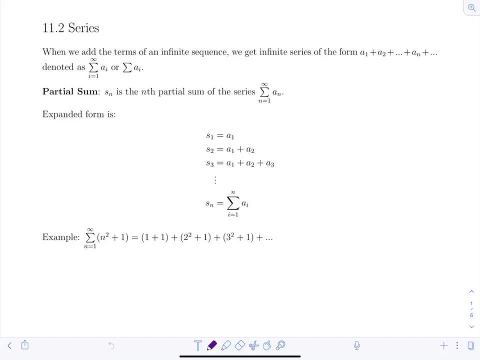 of the sequence, S3 would be the sum of the first three terms, and the pattern continues. So the nth partial sum consists of the sum of the first n terms. So here in summation notation this means my index of summation. i starts at 1.. So I take the first term and I sum up all the way up until 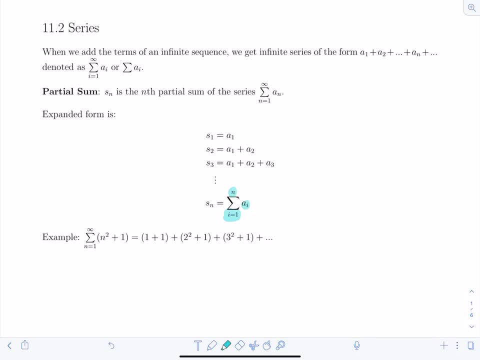 a sub n. Make sure, when you're representing this, you switch your index to i and you have a sub i, because n is reserved for the nth term, the last term. So this cannot have an n anymore. All right, let's look at an example to help us get more familiarized with this idea. So we have the 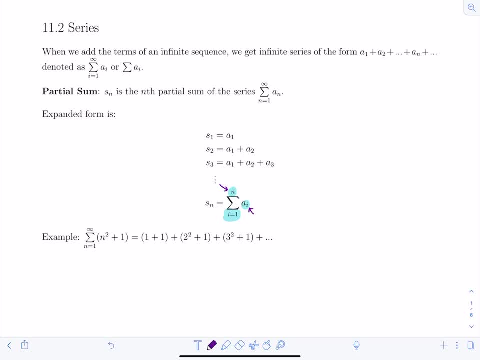 sum, infinite sum from n equals 1 to infinity of n squared plus 1.. So listing out the first few terms, If I substitute in 1 for n, I'd get 1 squared plus 1, that's the first term, that's a1.. 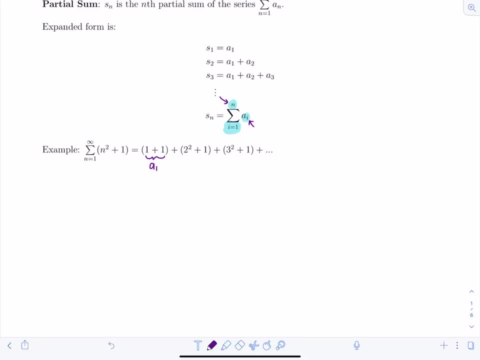 And then, since this is a series, then I'm going to add to it a2,, 2 squared plus 1, this is a3, etc. So s1, the first partial sum is just a1, which would be 2.. 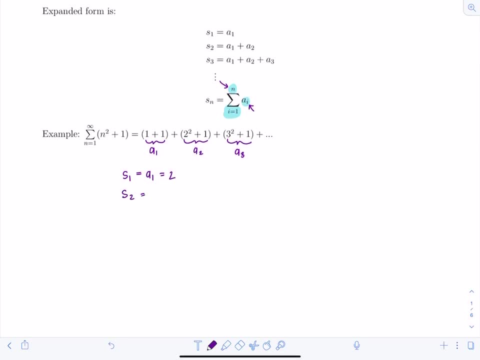 s2, the second partial sum is a1 plus a2, well, a1 was 2 and a2 is 5, so s2 is 7.. s3 is going to be. well, I can just take the previous partial sum and add the next term to it, right? 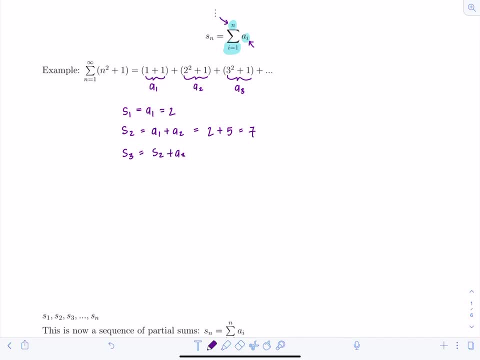 So s3 would be s2 plus a3, so s2 we have, that. it was 7. Plus a3. right here, 3 squared plus 1, that's 10.. So this is 17.. Let's do one more s4, that's s3 plus a4. 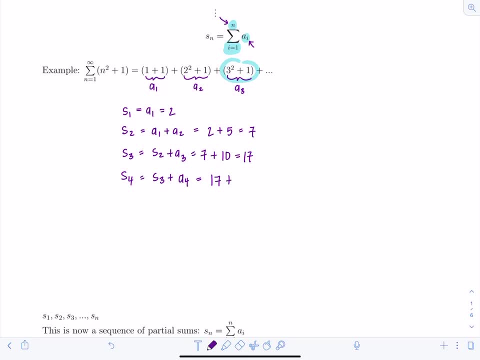 So that's going to be 17 plus, well, a4. we don't have it listed out here, but I can just get it by substituting 4 for n. So that's going to be 4 squared Plus 1, which is 17,. so 17 plus 17,, 34,, etc. 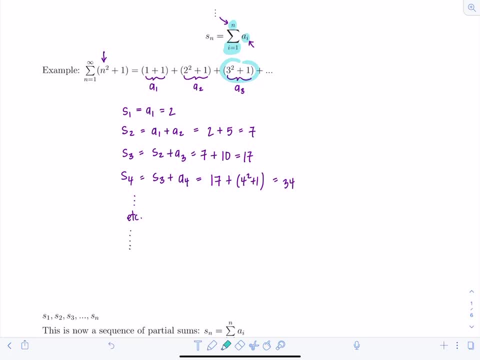 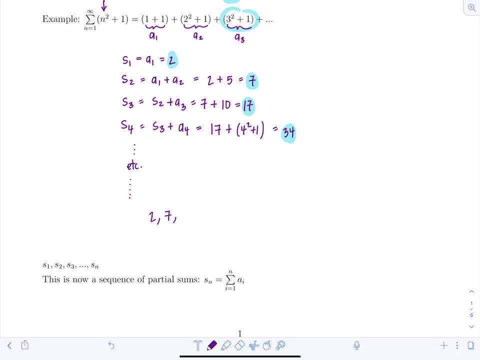 All right. and then notice here I could list these terms: s1 is 2,, s2 is 7,, s3 is 17,. s4 is 34.. Those make a new sequence: 2,, 7,, 17,, 34, and it continues forever. 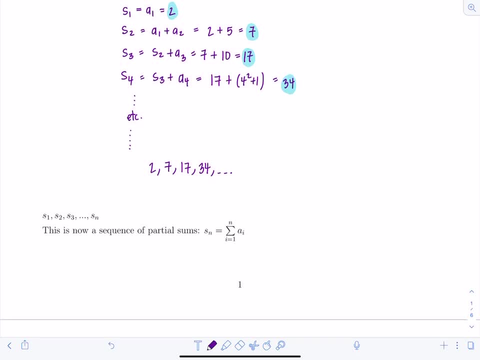 So, generally listing them out: s1,, s2, s3, all the way up to s, sub n. this is now a sequence of partial sums, So you can think of this as almost a new sequence that's built by adding up the terms from your original sequence, a sub n. 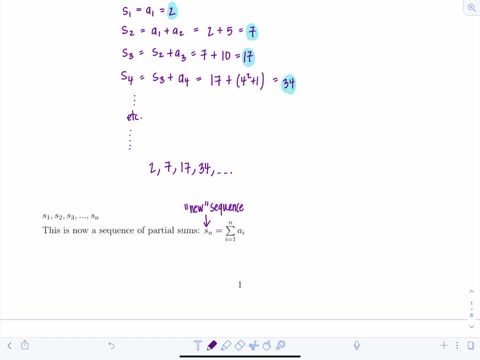 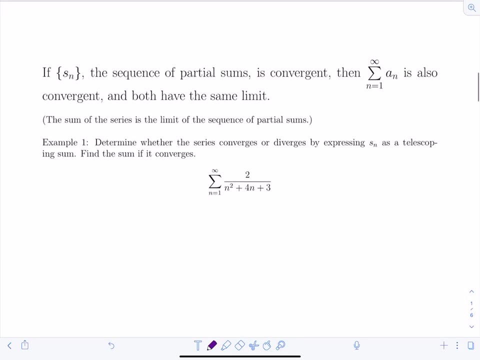 Okay. well, why are we talking about this sequence of partial sums? Well, because it gives us a lot of information about the infinite series. And here's the important part: If s sub n, the sequence of partial sums is convergent, 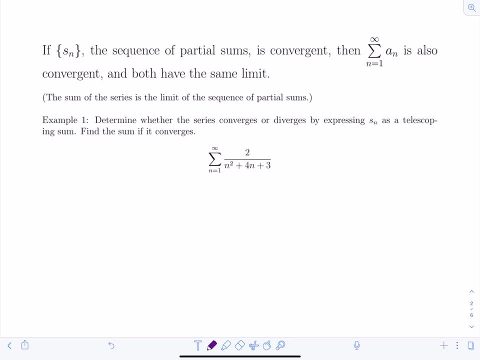 So if that sequence is convergent, then the infinite series from n equals 1 to infinity of a sub n is also convergent And they both have the same limit. So if the sequence of partial sums is convergent, then my infinite series or a sub n 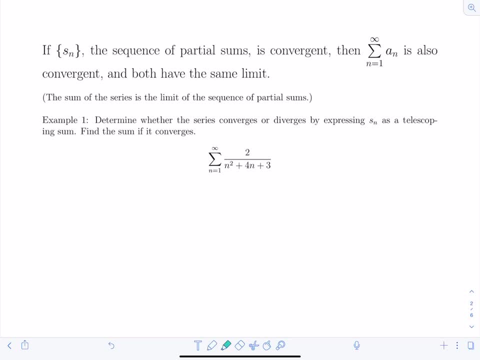 is also convergent And bonus. the sum of the series is equal to the limit of the sequence of partial sums. Now, this is very rare. In this chapter we're going to be studying and investigating the convergence of infinite series, And very rarely are we able to find out what the actual sum is. 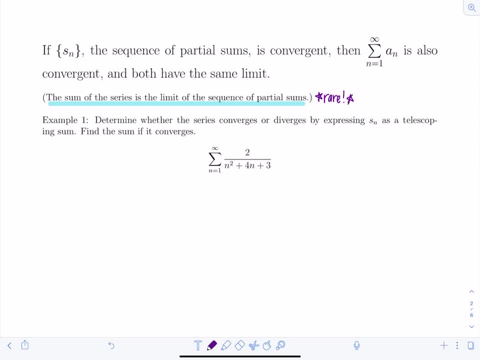 So this is one special case where, if we're able to evaluate the limit of the partial sums, the sequence of partial sums, then we do indeed have the sum of the series if it converges. Okay, so let's look at an example, Determine whether the series converges or diverges. 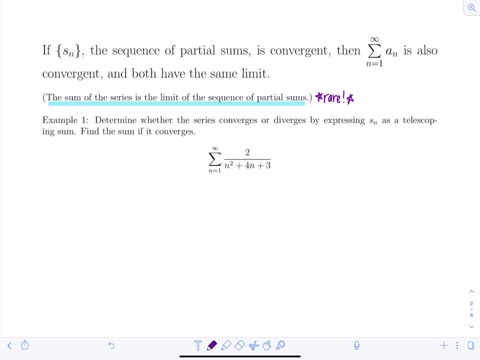 by expressing Sn, the sequence of partial sums, of the telescoping sum: Find the sum if it converges. So they're giving us a hint, They're telling us that this is a telescoping sum, And I'll show you exactly what that means. So let's first write out an expression. 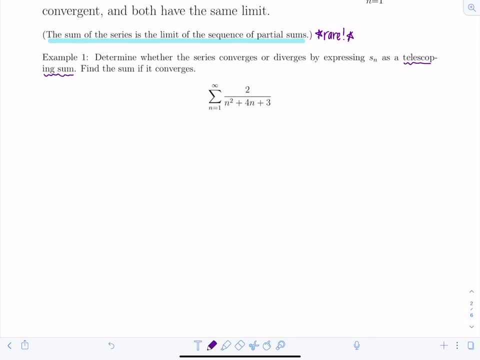 for Sn and then work with it from there. Now please have some caution here. Sn- the sequence of partial sums is the sum. Now I have to change my index. It starts from: i equals 1, up until n, n being the last or the nth term in this partial sum of the terms here. 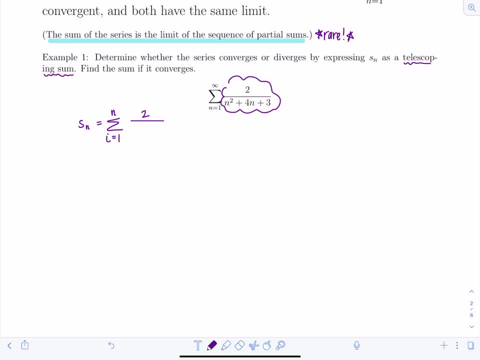 So this is going to be 2 over now. my index of summation is i, so I have to switch this to: i squared plus 4i plus 3.. You cannot have the same variable there as what the final term is going to. 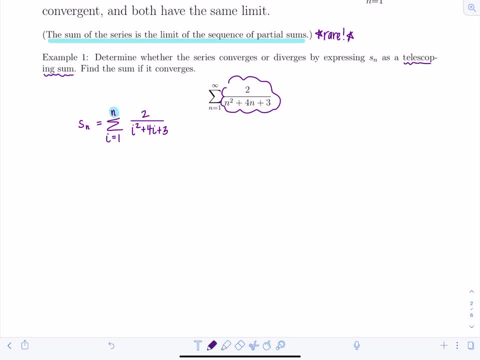 be. That wouldn't make any sense. All right, now I want to write this as a telescoping sum. So that means that when I'm expressing the sum of the terms, a lot of the terms in the middle are going to cancel out, and it's all going to cancel out. So I'm going to write this as a 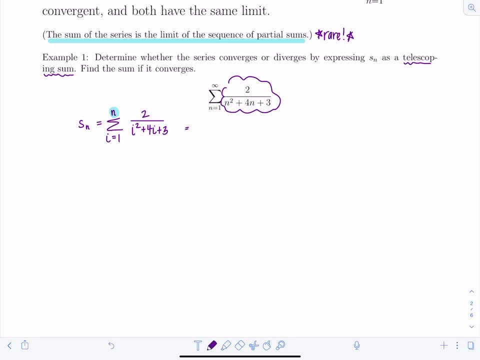 collapse, like a telescope collapses. So either you're going to use some partial fractions or some other techniques. We have another example after this, but I'm thinking let's do partial fractions because this denominator factors. So I can write this as i equals 1 to n of 2 over. 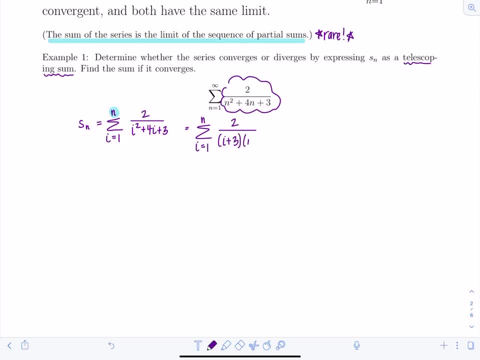 i plus 3 times i plus 1.. All right, and then, using partial fraction decomposition, I can rewrite this as: the sum i equals 1 to n of negative, 1 over i plus 3 plus 1 over i plus 1.. 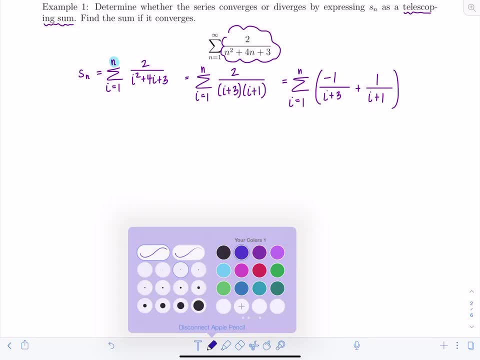 All right now. if you forgot your partial fractions, I'll just give you a little reminder here. So, aside, we have 2 over i plus 3 times i plus 1 equals a over i plus 1 plus b over i plus 3.. And then multiplying through by the LCD: 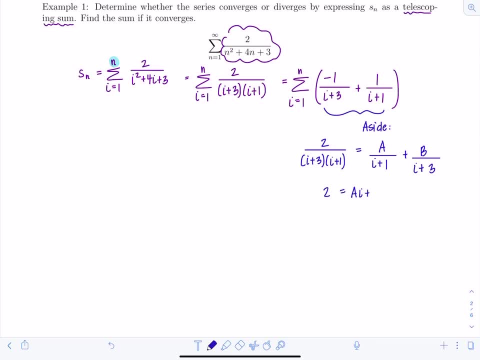 I would get 2 equals a, i plus 3, a plus b, i plus b, And then grouping my terms together, so a plus b must equal zero, because there's 2 and a plus i plus 1 in this same76今回offs 커 Duond тру Allied ofih hyung sam 베″h. 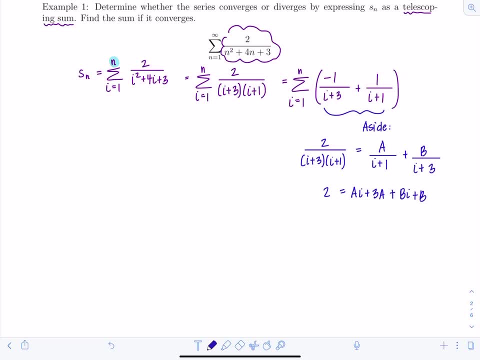 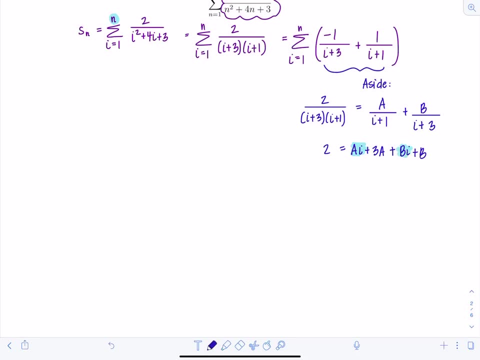 plus bi, plus b, AND THEN GROUPING MY TERMS TOGETHER, SO A PLUS B, MUST EQUAL ZERO, AND THEN GROUPING MY TERMS TOGETHER, SO A PLUS B, MUST EQUAL ZERO, AND THEN GROUPING MY TERMS TOGETHER SO A PLUS B, MUST EQUAL ZERO. 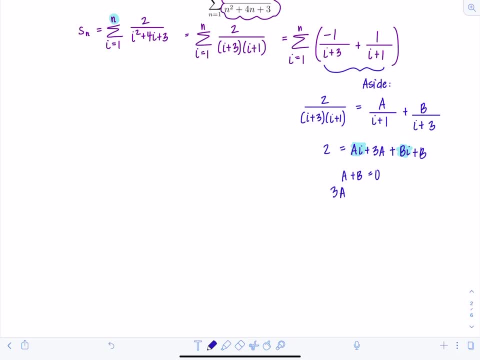 there's no, i's on the other side. And then 3a plus b, my constant terms equal 2.. I can subtract this top equation from the bottom. one b will cancel out, And I get 2a equals 2. That means a. 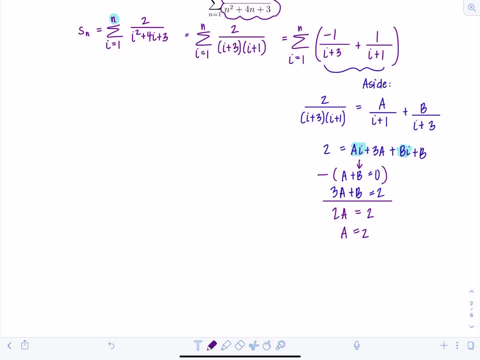 is 2.. And so if a is 2,, I mean a is 1.. So if a is 1, then b has to be negative 1.. All right, so there's our partial fraction decomposition. Now back to the problem. 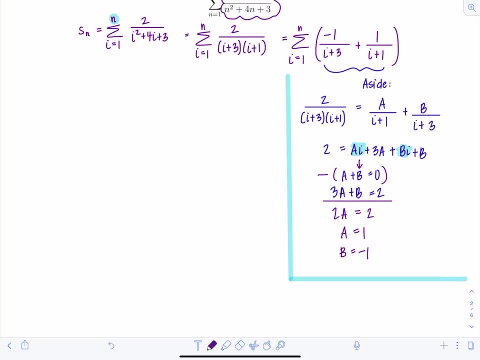 Okay, expressing this partial sum, So s sub n. I'm going to list out the first few terms. Okay, so I'm going to substitute in i equals 1 into the expression here. Okay so, substituting in i equals 1, I'm going to get negative 1 over 4.. 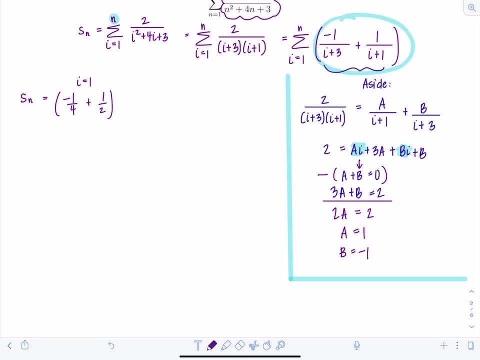 Plus 1 half. Okay, that's the first term Plus. now let's do. i equals 2.. So that would be negative: 1 over 5 plus 1 over 3.. Okay, let's keep going Plus. I don't see a pattern yet. i equals 3.. This is going to be. 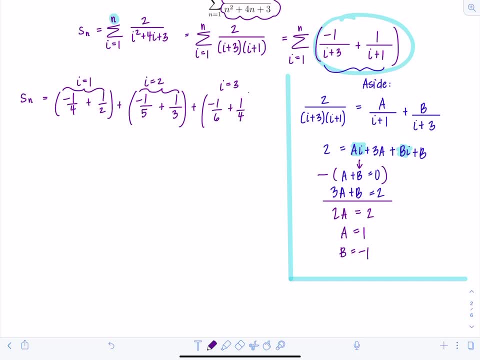 negative 1 over 6.. Plus 1 over 4.. Plus, let's do now: i equals 4.. So this is: i equals 4.. I'm going to have negative 1 over 7, plus 1 over 5.. Okay, now notice what's going on here. This is why it's called telescoping. 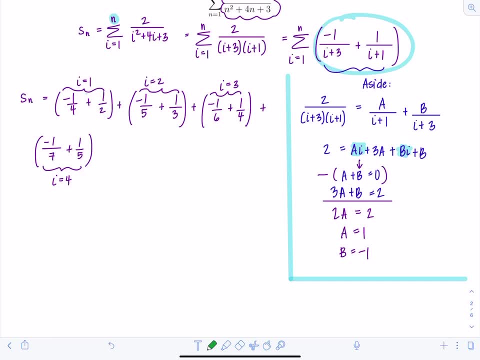 So I have this negative 1 fourth which is going to cancel out with the positive 1 fourth here. Also, I have this negative 1 fifth which is going to cancel with the positive 1 fifth here, And then, if I kept going, my next term I would be able to cancel out. 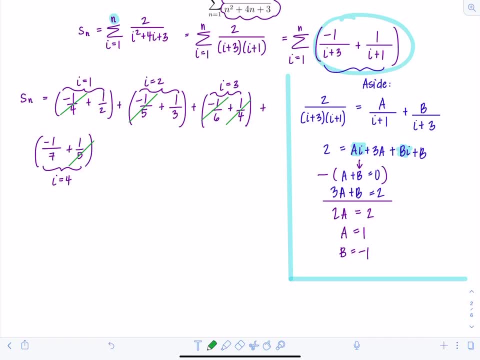 the negative 1 sixth. What would not cancel out? I mean, this negative 1 seventh would eventually cancel out, but nothing would cancel out with the 1 half or the 1 third. Those remain Okay. so we listed out the first four terms. I'm confident that the good rest in the middle are. 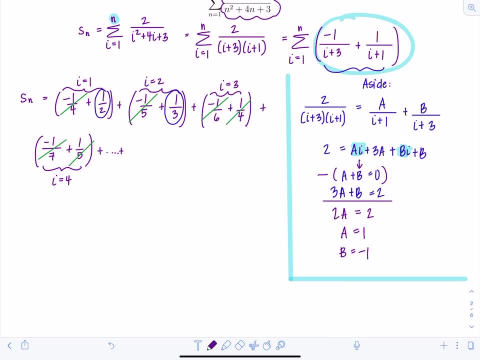 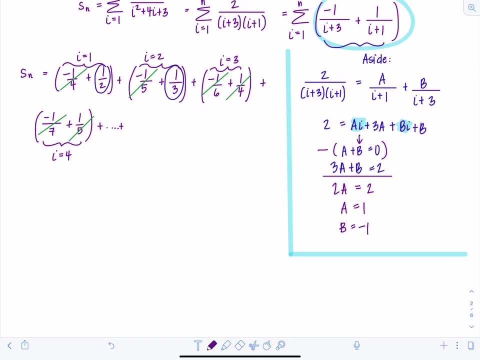 going to cancel out. Now let's see what happens for the last few terms. Okay, so, since I listed out the first four, the last term would be: i equals n. Before that would be i equals n minus 1, and before that would be i equals n minus 1.. And before that would be: i equals n minus 1.. 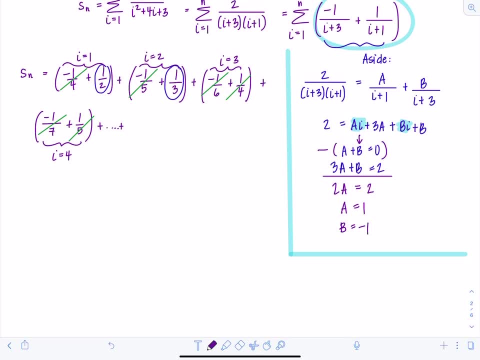 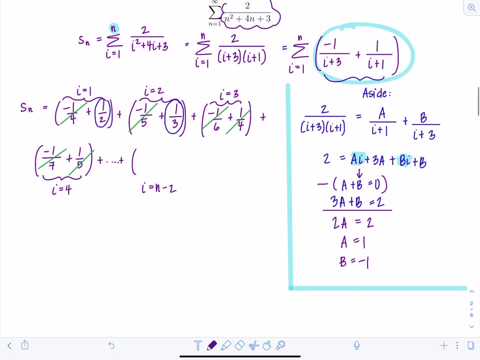 Before. that would be i equals n minus 2.. So let's list out. let's start with: i equals n minus 2.. All right, so if I substitute in n minus 2 for i, that's going to be n minus 2 plus 3 in the denominator. So that's negative 1 over n plus 1. 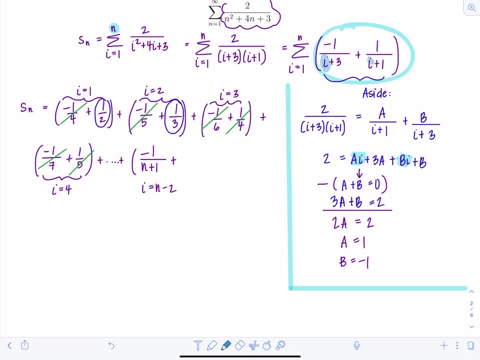 plus, And then again, if I'm substituting in n minus 2, here n minus 2 plus 1, that's going to be n minus 1.. So I have 1 over n minus 1 in the denominator. 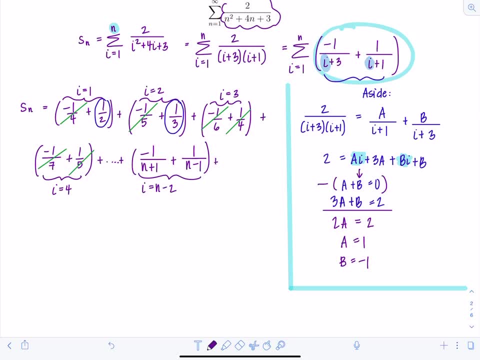 All right, what would come next? It would be: i equals n minus 1.. So same thing if I substitute n minus 1 into the denominator n minus 1 plus 3, that's n plus 2.. So I have negative 1 over n plus. 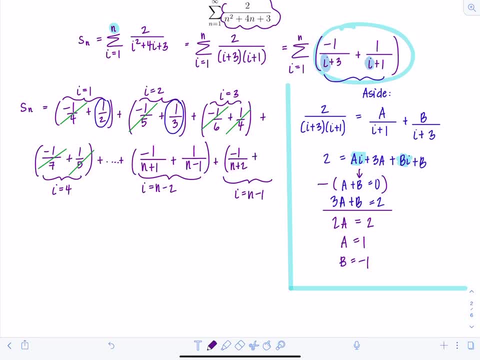 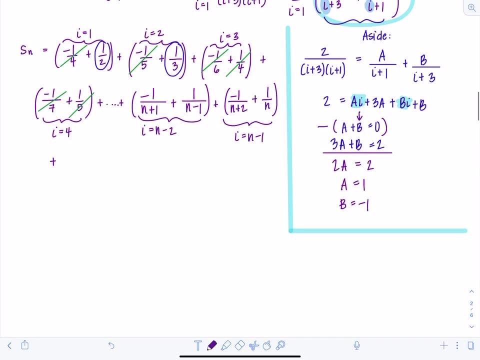 2 plus n minus 1 plus 1, that's just n. So 1 over n And then plus. let's do the last one: i equals n. So if i equals n, I would just have negative 1 over n plus 3 plus 1 over n plus 1.. So can you. 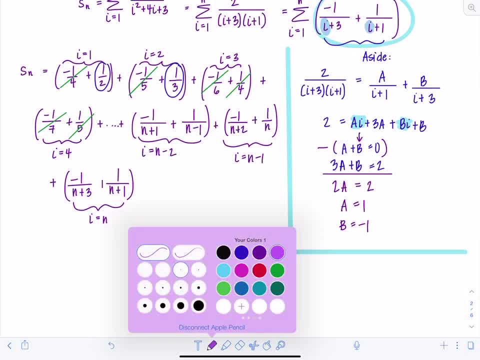 see what's going to cancel out. Well, this 1 over n minus 1 plus 1 is going to cancel out. This 1 over n plus 1 is going to cancel with the negative 1 over n plus 1.. And if I kept listing more terms, then the one prior would have the 1 over n cancel out, right. 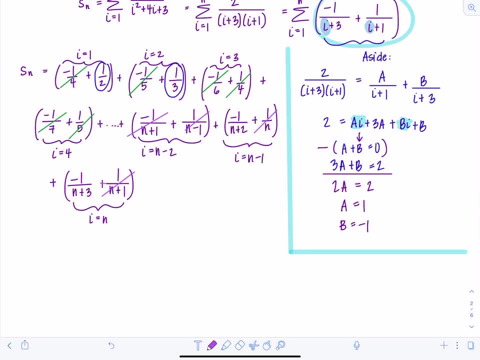 I'd have a negative 1 over n. This would cancel out eventually. What would not cancel out? Well, negative 1 over n plus 2 would not cancel out. Neither would negative 1 over n plus 3.. And you can always. 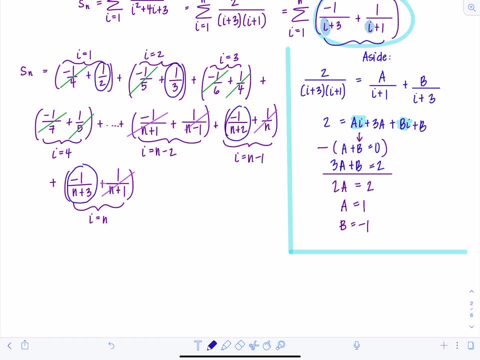 list more terms if you need, until you see a pattern. One thing that will always happen in a telescoping series is however many terms survive at the beginning in the first few terms. So in this case we had like two survivors that didn't cancel out. You're going to have the same. 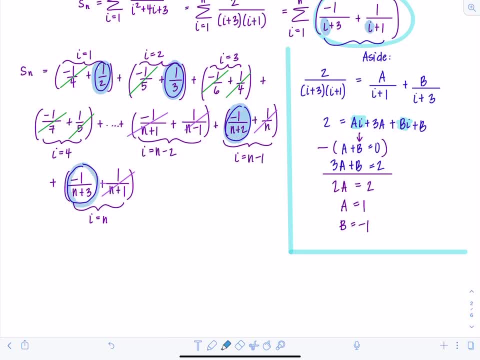 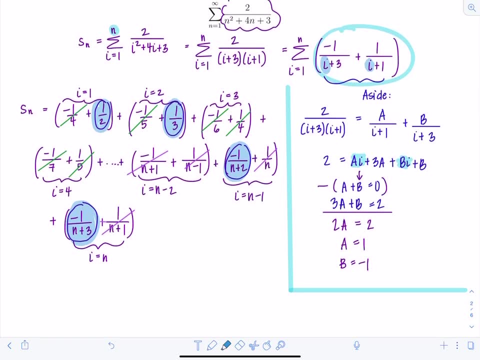 number at the end. Okay, And then also another thing to notice is that the denominators, when we have this partial fraction decomposition, they were i plus 3 and i plus 1, right, So those are two units apart. So that also comes into the picture. So you can see that the denominator is. 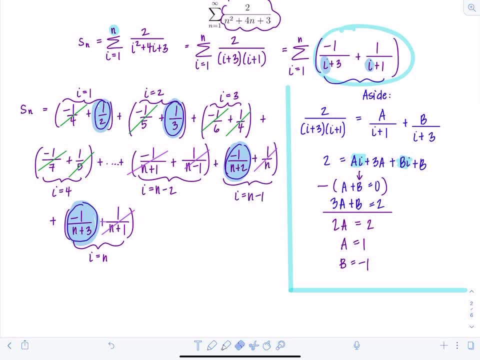 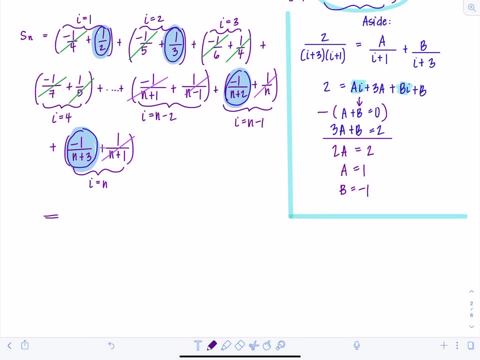 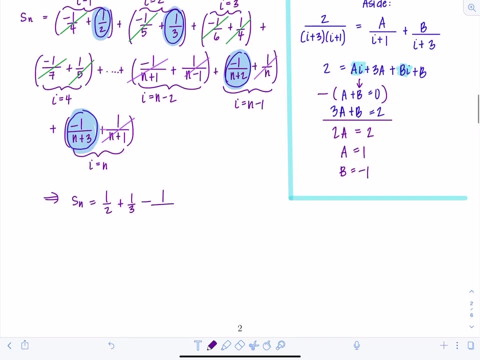 to play with the fact that there were two terms in the beginning and two at the end. that didn't cancel All right. so now I can rewrite Sn as 1 half plus 1 third minus 1 over n plus 2 minus 1 over n plus 3.. And remember now, if I want to figure out whether or not my series or my sum, 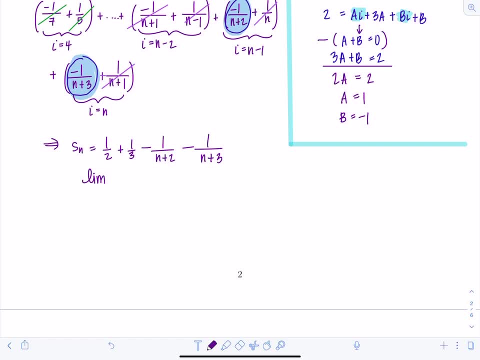 converges or diverges. I'm going to take the limit as n approaches infinity of Sn. So that's going to be the limit as n approaches infinity of 1 half plus 1 third minus 1 over n plus 2, minus 1 over n plus 3.. Now, if n goes to infinity, 1 half and 1 third are constants. 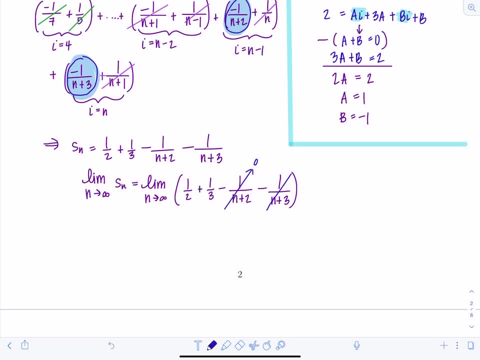 The other terms go to 0, since we have a constant over n. So I'm just left with 1 half plus 1 third, which is 5 over 6.. So since that limit exists as a finite number, I can say my series converges- Very exciting. And in fact this is the sum. 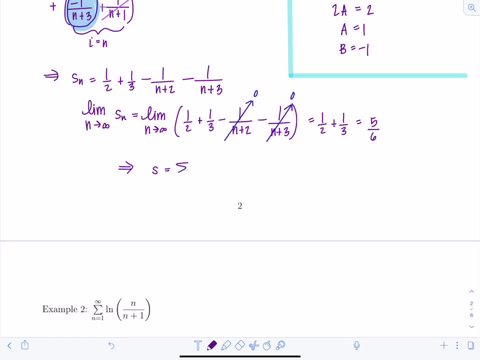 So I can write S as in the sum of my series. write what the original series was: n equals 1 to infinity of 2 over n, squared Plus 4n plus 3. This equals 5 over 6. And therefore it converges. 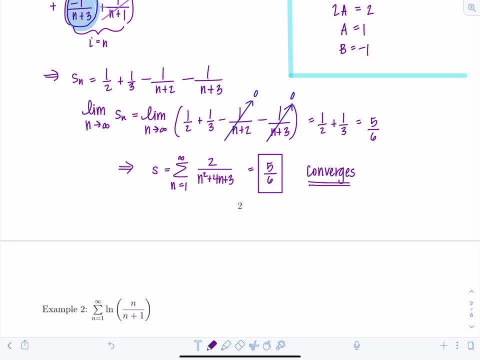 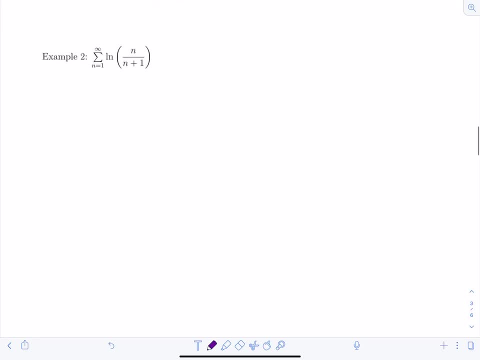 Okay, nicely done. Let's look at another example of a telescoping series. In this case we have a natural log. So we have the sum n equals 1 to infinity of the natural log of n over n plus 1.. So first I'm going to write S as 1 half plus 1 over n, plus 2 minus 1 over n squared. 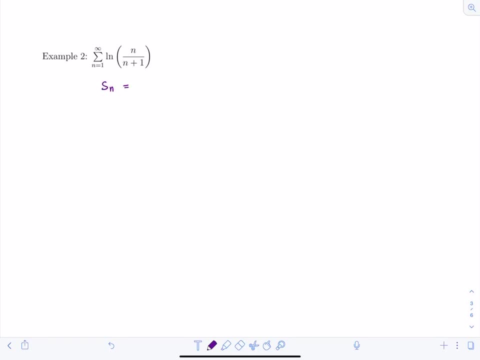 So I'm going to write an expression for S sub n. So we have the sum. Remember, change your index to: i equals 1 to n of the natural log of, and change it here as well: i over i plus 1.. All right If. 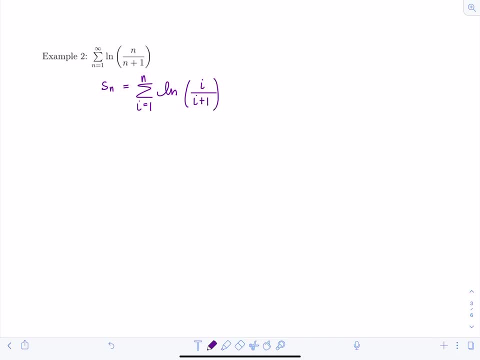 your notation is not perfect, it is considered incorrect and you'll lose points. Now from here, remember, for telescoping we wanted to have terms cancel out when we were adding them together, So I need some sort of addition or subtraction to go on. That's why last time we did the 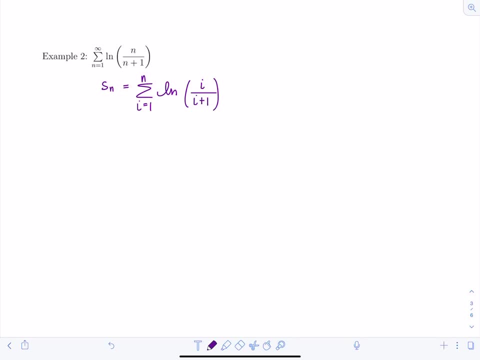 partial fractions. Well, this time I'm going to use my properties of logarithms So I can rewrite natural log of i over i plus 1 using subtraction. So this is the sum i equals 1 to n. natural log of i minus natural log of i plus 1.. All right, So let's start listing out the first few terms. 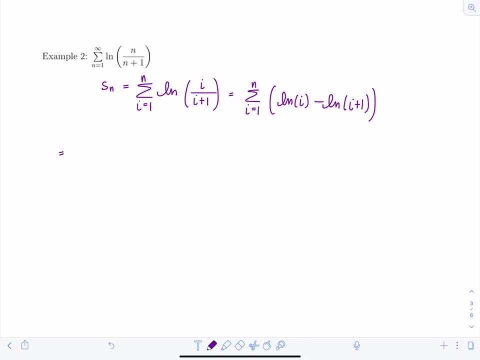 So if I substitute in 1 for i, I'm going to have natural log of 1 minus natural log of 2.. So this is for i equals 1.. Plus now for i equals 2, I'm going to have natural log of 2 minus natural log of 3.. 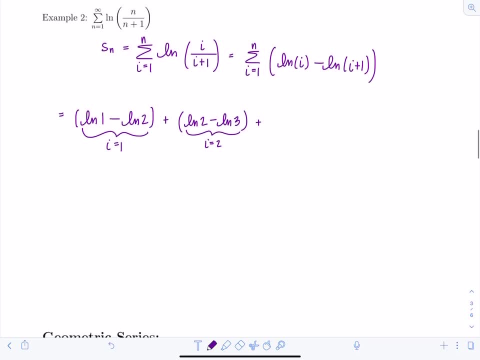 Plus, let's keep going until you feel comfortable that you see a pattern. Let's substitute in: i equals 3.. We have natural log of 3 minus natural log of 3.. All right, Do we see any patterns emerging? Well, first things first, natural log of 1,. 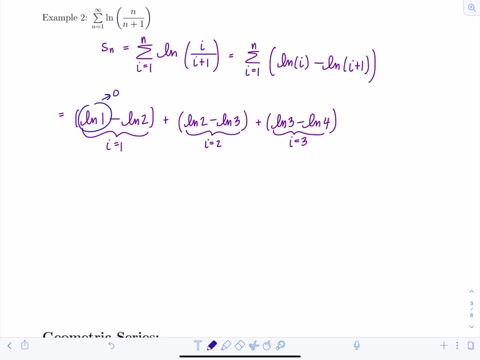 that's just 0.. And then here already, things are canceling out. So ln of 2s cancel out. ln of 3s cancel out, Wow OK. So technically, the only one that didn't cancel was this ln of 1,. 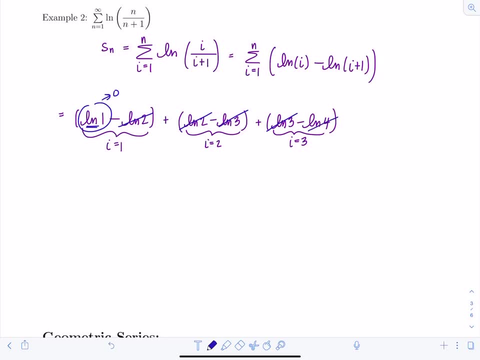 which is 0. Because in the very next one, ln of 4 would cancel out right, Plus dot, dot, dot. And then let's start at the last n. So we're going to have natural log of 1 minus natural log of 2.. 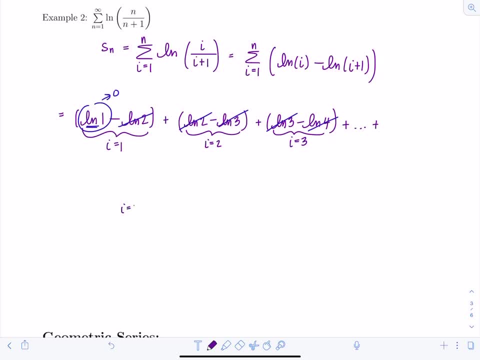 Let's do the last 3, like last time, So we can do. i equals n minus 2.. So we would have ln of n minus 2 minus ln of n minus 2 plus 1 is going to be n minus 1.. 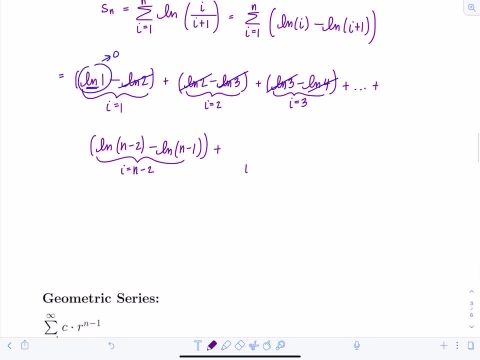 Plus, And then next one we'll do: i equals n minus 1.. So this would be ln of n minus 1, minus natural log of just 1.. n, this time plus, and then last one: i equals n. we'll have natural log of n. 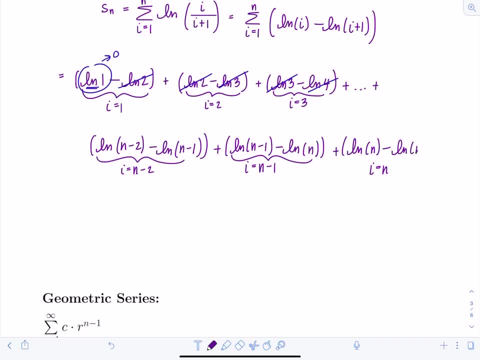 minus natural log of n plus 1.. That's for i equals n. Okay, so do we see any cancellation? Definitely, So ln of n is gone. ln of n minus 1 cancels out, And then I know, ln of n minus 2. 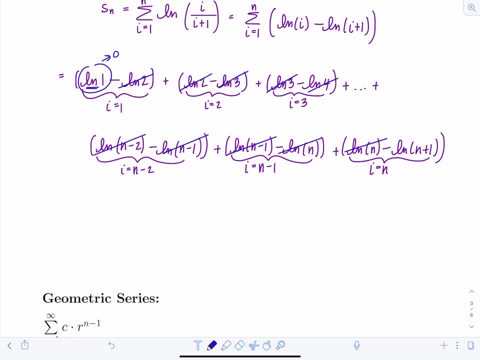 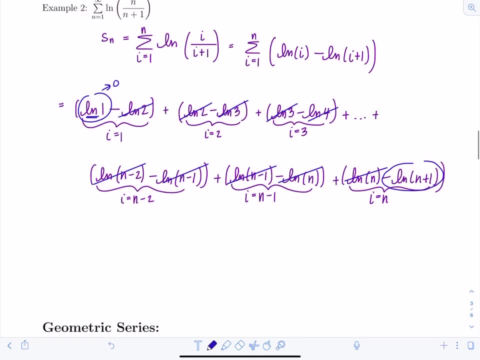 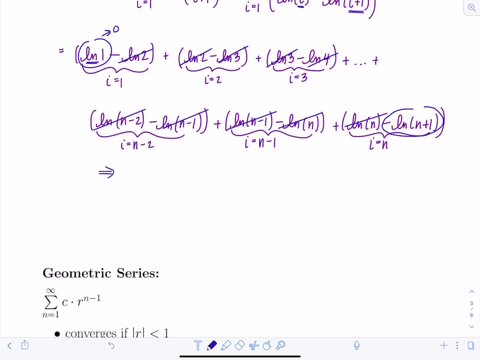 would cancel out. right, for i equals n minus 3.. So the only term that survives is the last one, just like the first one did here. one on each side, And I expect that because the difference here is just by one. All right, so now this means S sub n see how it telescopes everything. 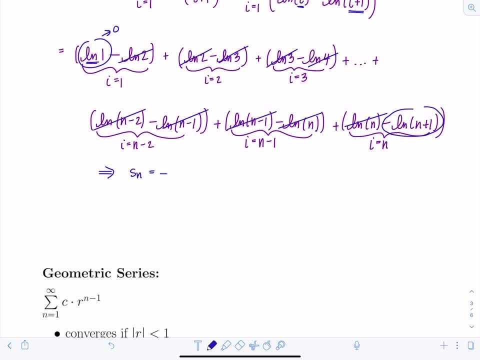 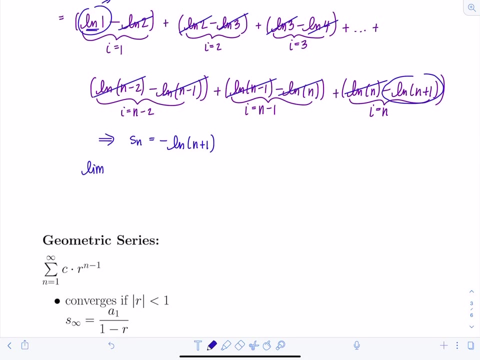 collapses in the middle. So S sub n equals the negative natural log of n plus 1.. So now, in order to determine whether or not the series is convergent or divergent, I need to take the limit as n goes to infinity of S sub n. So the limit as n goes to infinity of S sub n is equal. 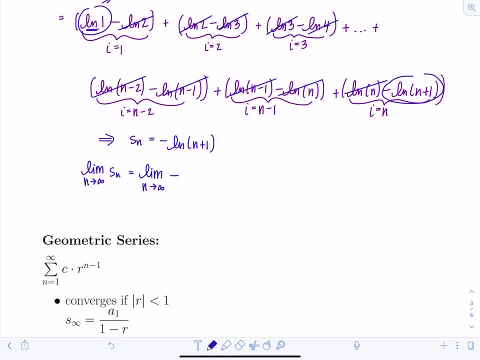 to the limit, as n goes to infinity, of negative ln of n plus 1.. Well, what's this limit going to be? Well, imagine the graph of natural log. right as n approaches infinity, natural log approaches infinity. And then, since I have that minus sign, this is going to approach. 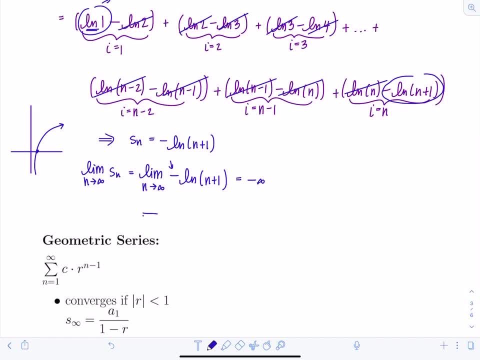 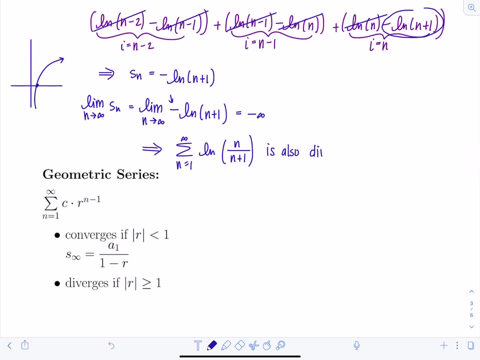 negative infinity. So what does that tell me? That's not a finite number. Therefore, my series n equals 1 to infinity. natural log of n over n plus 1 is also divergent. All right, that means it does not sum up to a finite number. 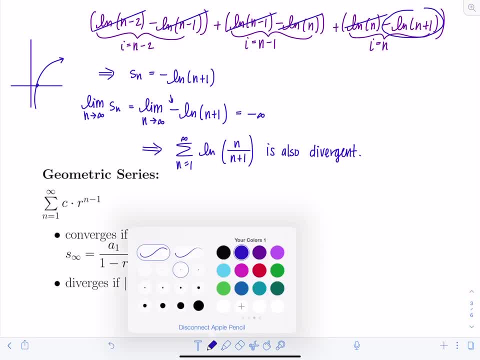 I want you to notice something, though: The infinite series is divergent. What are the terms? What's the sequence of those terms, though A sub n is natural log of n over n plus 1.. Now, last section. we looked at the limits of sequences, So the limit as n approaches infinity. 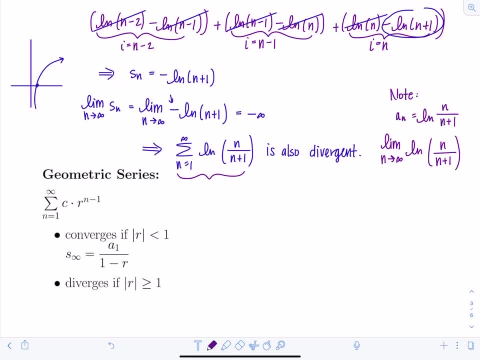 of natural log of n over n plus 1, well, natural log of n over n plus 1 is also divergent. Well, natural log is continuous, so I can pass the limit through. So I have natural log of the limit as n approaches infinity, of n over n plus 1.. This is going to approach 1.. 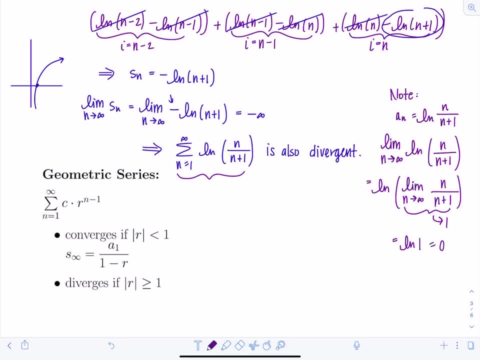 So this is natural log of 1, which is 0. So the limit of the terms is 0. But the sum, that infinite series, that does not converge. So we're going to study that interesting scenario a lot more throughout the chapter. 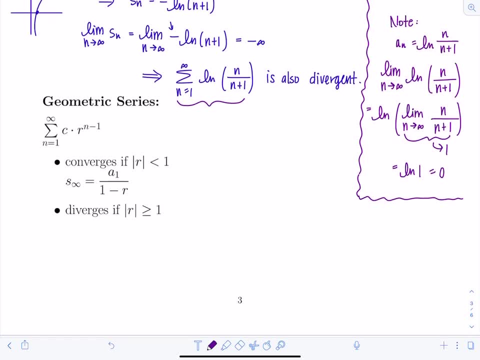 OK, another kind of series which are fairly easy to test, whether or not they converge or diverge, are geometric series. So remember, geometric series are ones that have a common ratio, R, meaning that to get from one term to the next, 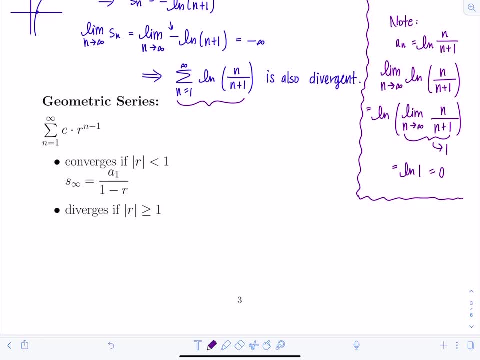 you're multiplying by R by some constant And we express an infinite geometric series in the form: sum of n equals 1 to infinity, of c times R to the n minus 1.. And it as long as the absolute value of r is less than 1.. Basically that would mean that term to term, 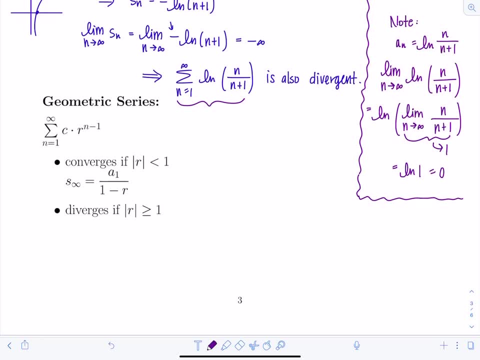 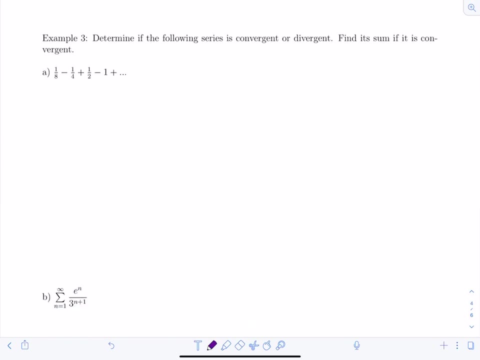 is shrinking right, Because you're multiplying by a fraction And we can compute that infinite sum as a sub 1, so the first term divided by 1 minus r, It diverges otherwise. okay, That's great. So now let's determine whether or not the following series is convergent or: 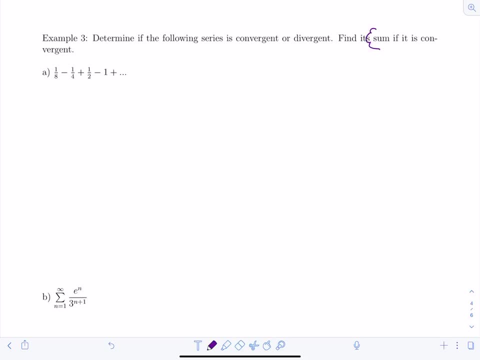 divergent, Find its sum. if it is convergent, Again, it's super rare to be able to find the sum. So really treasure this section because this is special stuff- Telescoping and geometric- that's when you can find the sum, All right, so let's look here: 1 eighth minus 1. fourth plus 1. 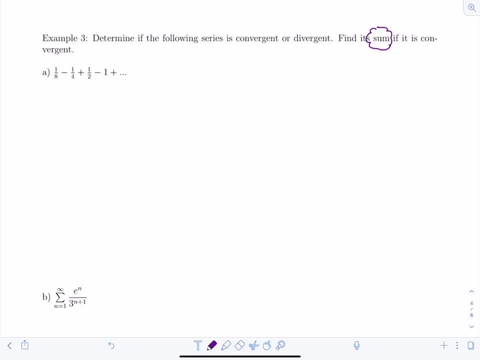 half minus 1.. So it looks like it's geometric. In order to find r, all you need to do is take one term and divide it by the term that proceeds. So r equals negative 1 fourth over 1 eighth And that's going to be negative 2.. And if it's a true geometric series, that r is going to be. 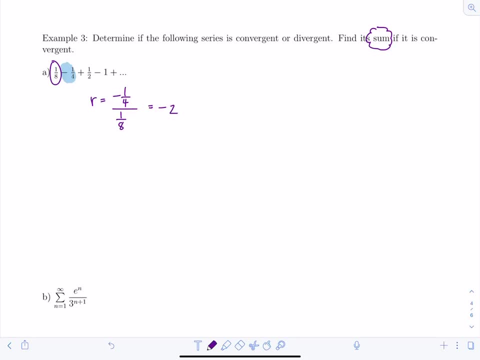 constant from term to term. So it doesn't matter which 2 you divide, You just take 1, divide it by the term. that proceeds it. Well, our test is pretty straightforward: Absolute value of r is going to be the absolute value of negative 2, and this is greater than 1.. 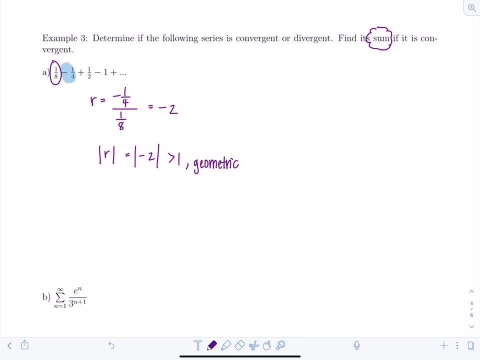 So since this is a geometric series and r absolute value of r is greater than 1, that means it diverges And we're done. So I can't find its sum. It doesn't have a finite sum. Great, next one. we have the sum. n equals 1 to infinity, e to the n over 3 to the n plus 1.. 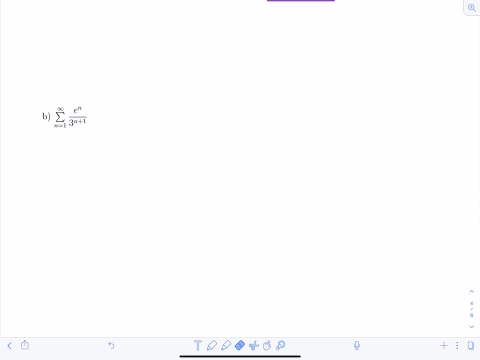 So this is already written in summation notation. I just have to figure out how I can rewrite the expression for the series so that I can identify what r is. So notice a sub n. the terms are represented by e to the n over 3 to the n plus 1.. So I can rewrite the 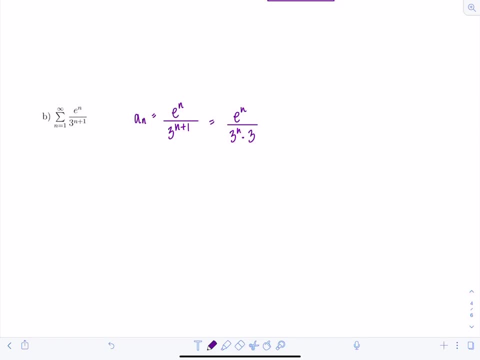 denominator as 3 to the n times 3 to the first right. And then now I can regroup things so that I just have the 1 third times e divided by 3 to the n. So whatever quantity is being raised to the n, that's your r right there. So this tells me. indeed, this is a geometric series. 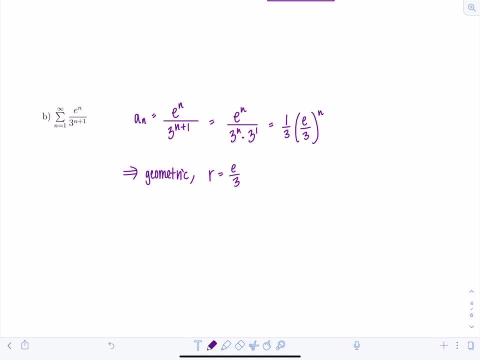 r is equal to e over 3 and the absolute value of r is equal to the absolute value of e over 3.. And we know e is about 2.7.. 2.7 divided by 3, that's going to be less than 1.. 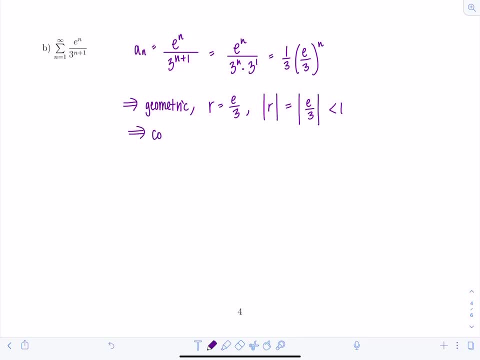 So this tells me my series is convergent, So I can regroup things. So I can regroup things. So if I want to find its sum, since I know it converges and it's geometric, I have a lovely formula: a sub 1 over 1 minus r. When you just see s written this way, that means the infinite sum. 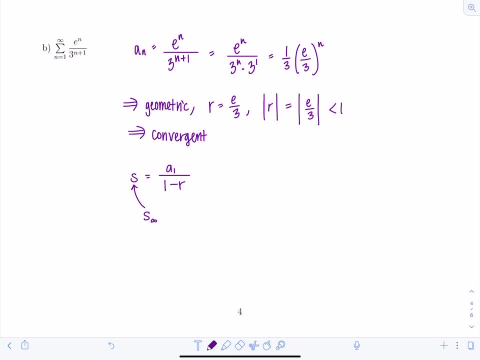 okay, If it's a sum of a partial sequence, it's going to have an index at the bottom telling you where it's stopping. So this equals a sub. 1 is the first term, So if I plug in 1 for n here, 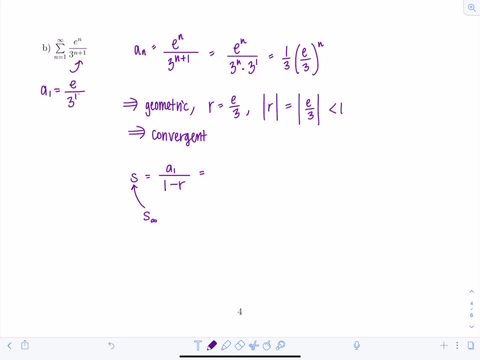 I'm going to have e over 3 to the 1 plus 1, or 3 squared, so that's e over 9.. So a1 is e over 9 over 1, minus e over 3.. Then I'm going to multiply everything. 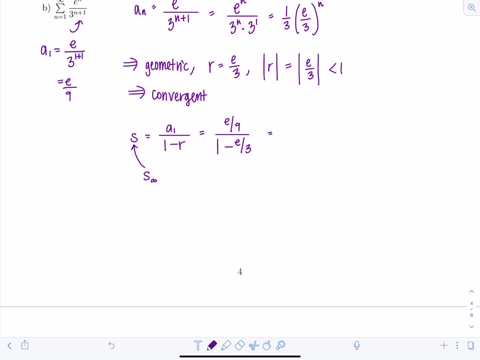 through by 9.. So I clear out the fraction. So we're going to have e over 9 minus 3e And I can factor out a 3 from the denominator, So I have e over 3 times 3 minus e. 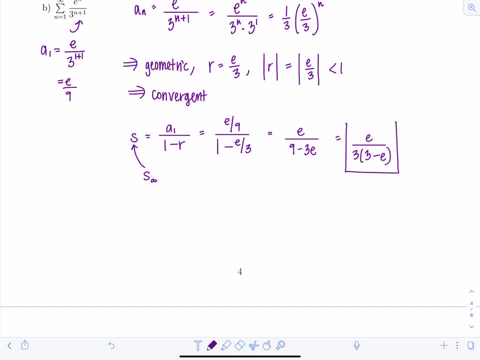 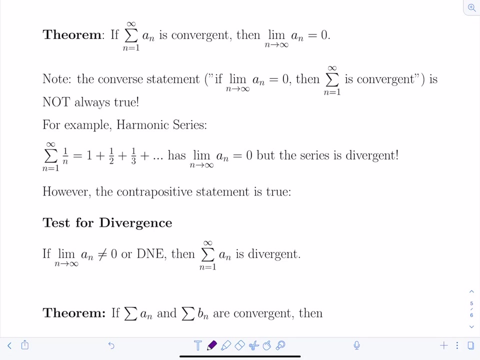 So I have a convergent geometric series And here is its sum. All right, All right, Nice. Now some very exciting theorems. First theorem tells us: if the sum n equals 1 to infinity of a sub, n is convergent. so if my infinite series is convergent, then the limit 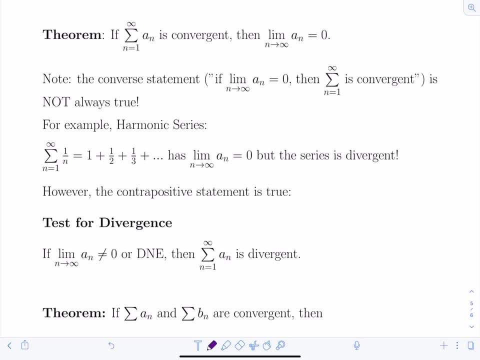 as n approaches infinity of a sub, n is 0. That means the terms go to 0. If I know my series converges, then the terms go to 0.. Notice the converse statement: If the terms go to 0, if the limit as n approaches infinity of. 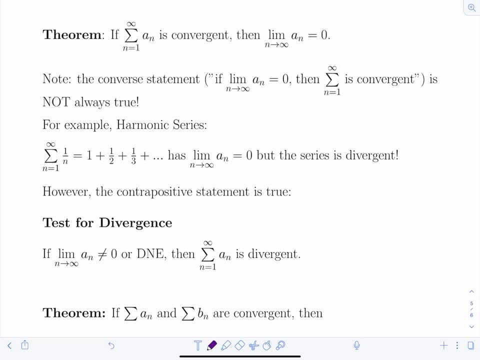 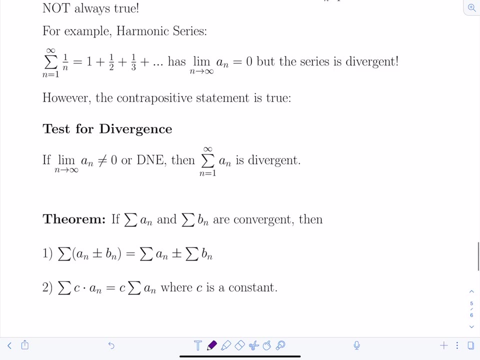 a sub n is 0, then the series is convergent. That is not true, necessarily. OK, I need an a sub n here, For example. most classic example of where this fails is the harmonic series. So the harmonic series is so famous it has its own little name. So it's the sum n equals 1 to infinity, of 1 over. 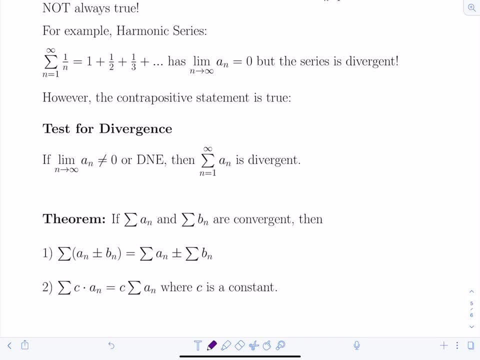 n. So if you list out the first few terms, it would be one plus a half plus a third, etc. And the terms go to zero. right? The limit: as n approaches infinity of a sub n of one over n, that limit is zero. 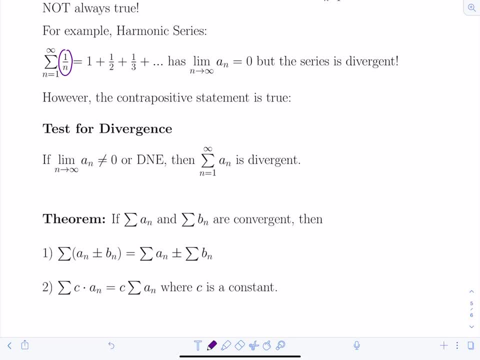 But the series is divergent. Why is that? Well, even though the terms are going to zero, even though the terms are shrinking, they're not shrinking fast enough so that, when you're adding them up, that sum approaches a finite number. 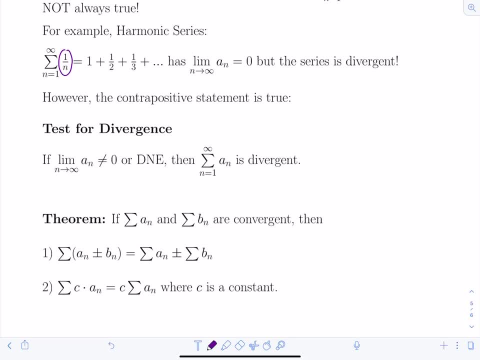 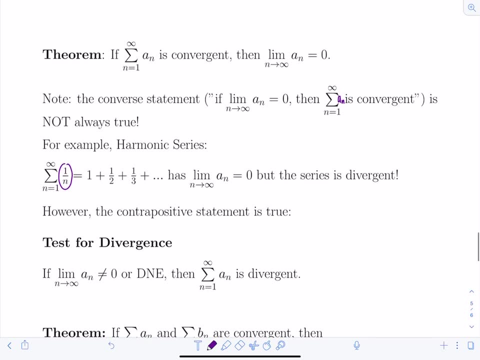 So they're shrinking, but just not quickly enough. Keep that in mind. However, the contrapositive of the theorem above is true, right. Anytime you have a statement, a true statement, it's contrapositive is always going to be true. 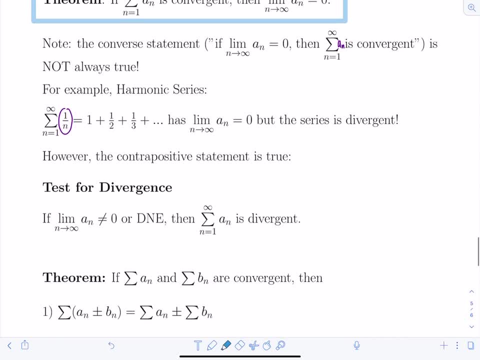 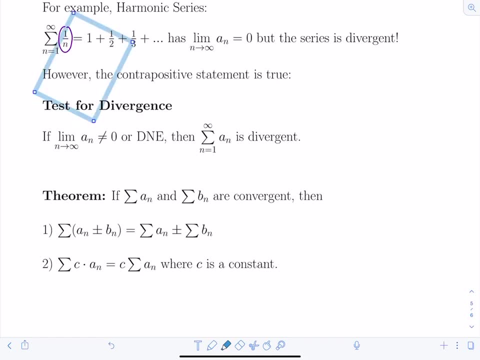 And the contrapositive of this theorem is the test for divergence. So the test for divergence tells us if the terms of a series- oh so if the limit as n approaches infinity of a sub n does not equal zero, or if it does not exist. 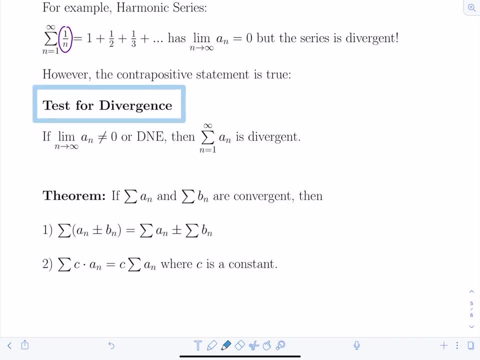 then I know my series, or the sum n equals one to infinity of a sub n is divergent. So basically, if these terms aren't going to zero, there is no chance that you're going to be able to add them up forever and have your series converge or approach a finite number. 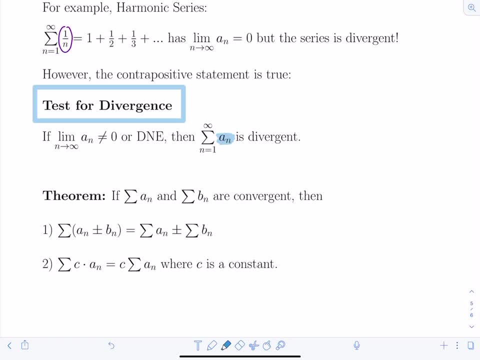 And you should always, if you're being asked to test for convergence or divergence of a series, run the test for divergence, at least mentally, before you get going. okay, Throughout the chapter you're going to learn many different tests for convergence or divergence of a series. 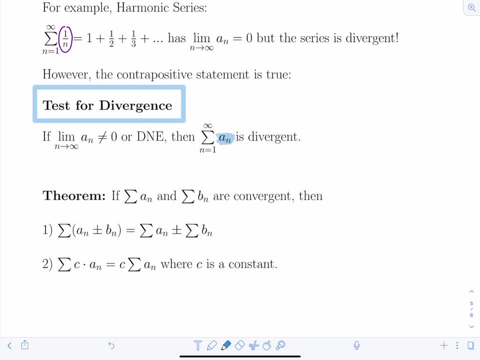 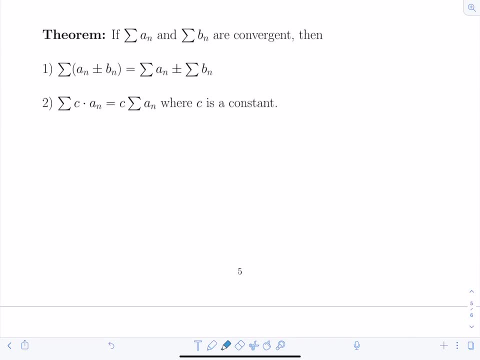 and this is one you want to always check first. Okay, a couple more theorems. If you have two series that you know are convergent already, so if the sum of a- n and the sum of b- n are both convergent, 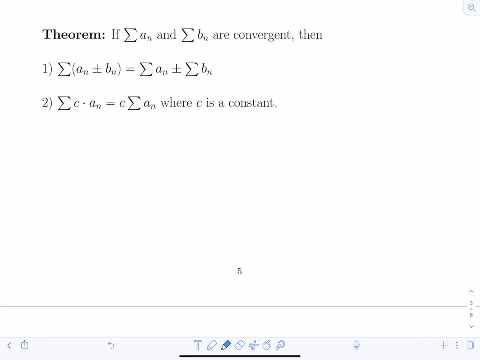 then you are allowed to distribute the summation across addition and subtraction And you're allowed to multiply through and take a constant outside of the sum. However, if you do not know that your series a, n or b? n are convergent to begin with, 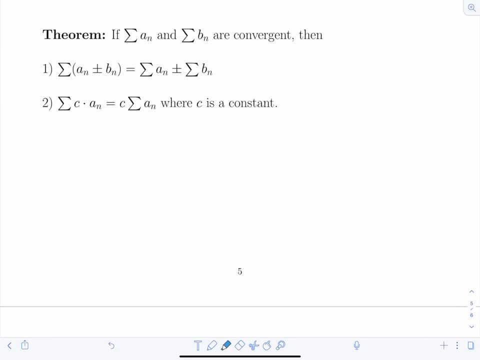 then you are not allowed to do the following, And it may seem a little strange because normally we think addition and subtraction are associative, but series are a lot more tricky or high maintenance of quantities to deal with. And just an example to drive this point home: 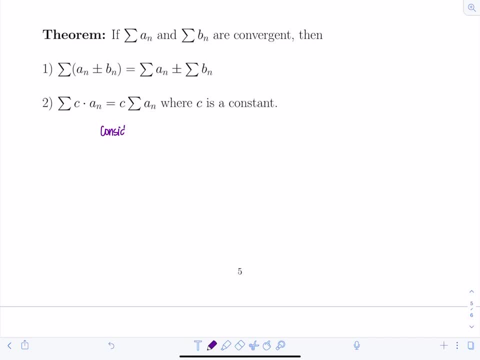 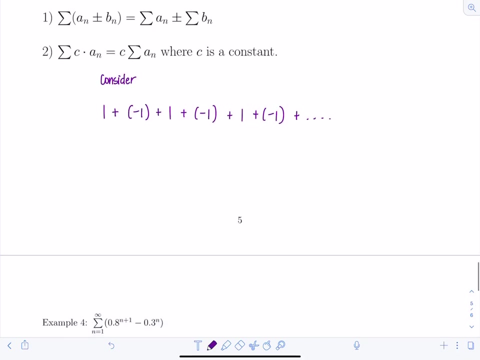 So say you have the series. let's consider 1 plus negative, 1 plus 1 plus negative, 1 plus 1 plus negative, 1.. It just goes on like that. okay, Is this series convergent? Well, you have to ask yourself: is the sequence of partial sums, is that sequence convergent? 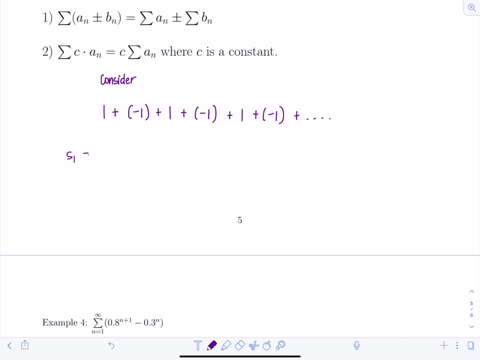 Well, what would the partial sums be? So the first partial sum- s1, would just be the first term, which is 1.. The second partial sum would be the sum of the first two terms. So 1 plus negative 1, that's 0.. 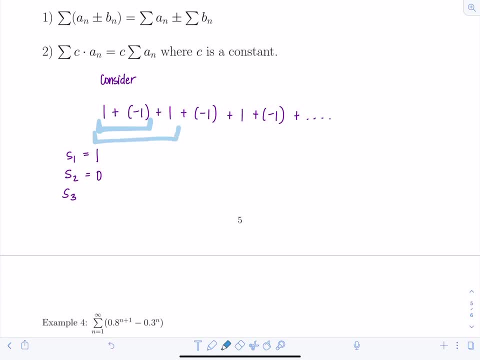 S3 would be the sum of the first three terms, So 0 plus 1,, which is 1.. s4 is 0.. s5 is 1, etc. Now look, is this sequence here convergent? Does it have a limit? 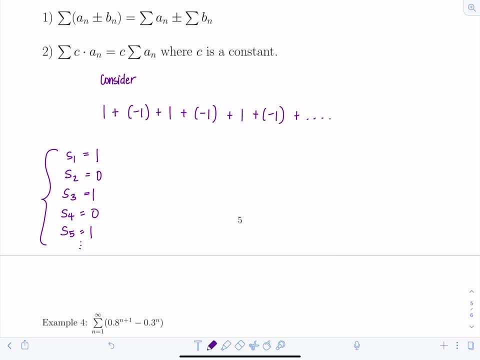 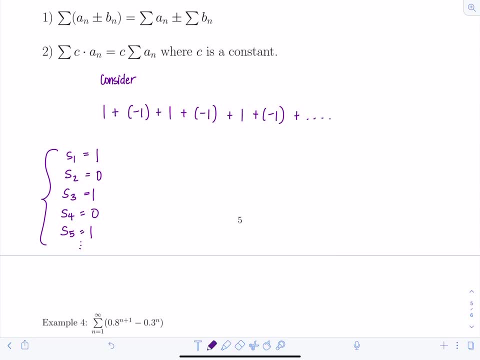 one and zero. However, now here's where things can get dangerous If I introduce grouping symbols. so if I group these two terms together, if I group these next two terms together, if I group these two terms together now, I'm changing the order of operation. So I would 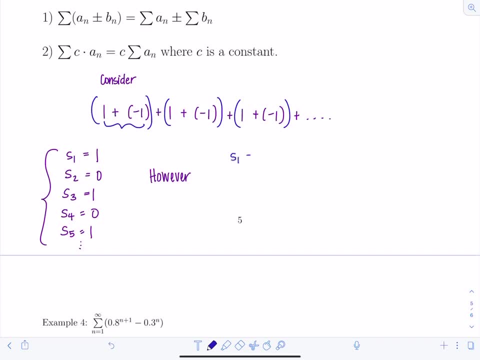 add those two together, one and negative one, So S1 would be zero. This sum is also zero, So S2 would be the sum of zero plus zero, which is zero. S3 would be zero plus zero plus zero, which is zero. So in this case it is convergent. 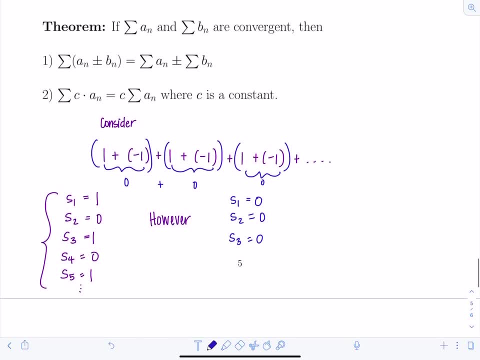 That's why you have to be careful that you do not distribute summations across addition or subtraction. You have to be careful that you do not distribute summations across addition or subtraction unless you know that these two series are convergent to begin with. Okay, so watch as I work through the next examples, because I'm going to do so very. 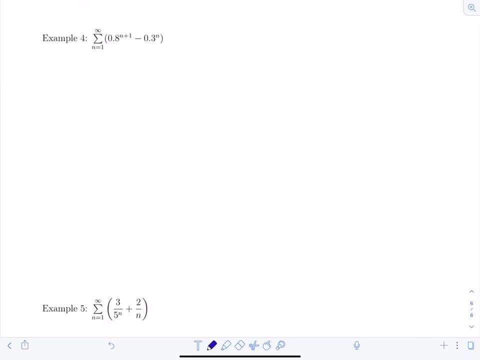 carefully and methodically, and you need to do the same. All right, so we have: the sum n equals one to infinity, 0.8 to the n, plus one minus 0.3 to the n. So I want to determine whether 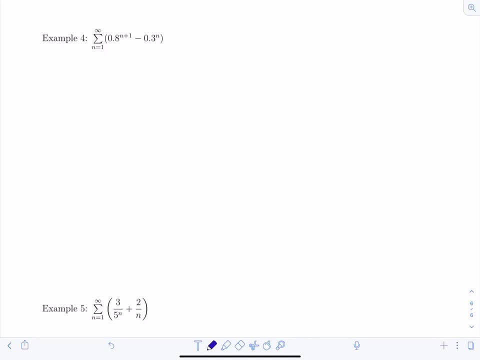 or not, it's convergent or divergent, and if it's convergent, find the sum. So I'm going to consider each of these series separately. So I'm just going to consider the sum. n equals one to infinity, of 0.8 to the n plus one. 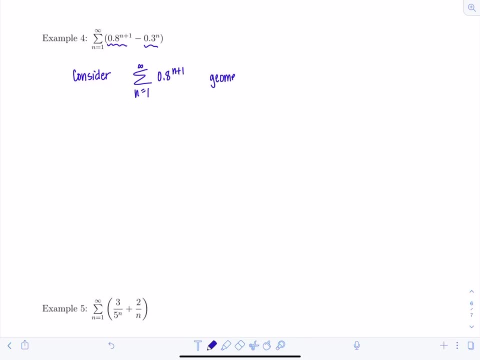 Okay now, what can I say about this series? Well, it's clearly geometric. r equals 0.8, and the absolute value of r is absolute value of 0.8,, which is less than one. So that means that series converges. I can find its sum. Its sum is a1,. 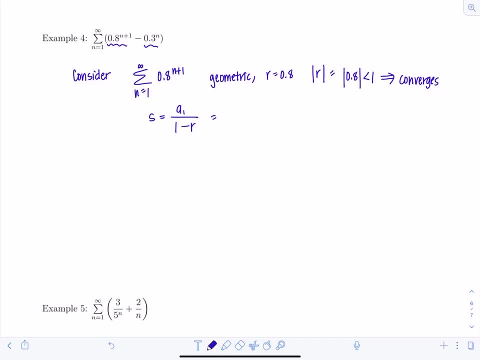 over one minus r, So a1,. if I substitute a1 for n, that's going to be 0.8 squared so 0.64, over one minus 0.8.. So 0.64 divided by 0.2, that's going to be 3.2.. 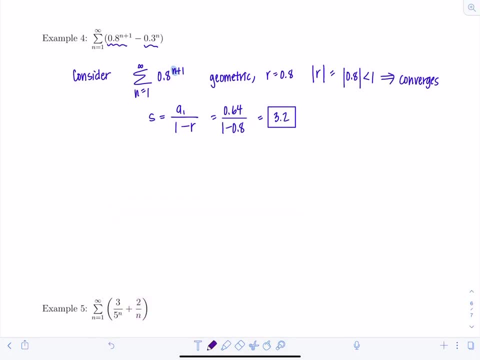 Okay, now let's separately consider Another geometric series. the sum n equals one to infinity, of 0.3 to the n. This is also geometric. r equals 0.3, and the absolute value of r- that would be the absolute value of 0.3, is less than one, which tells me it also converges. 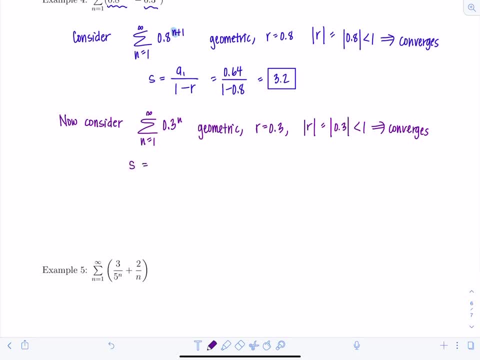 Okay, I can find its sum right. I have a nice formula for geometric series, So the first term would just be 0.3 to the first, so 0.3, over one minus r, one minus 0.3.. 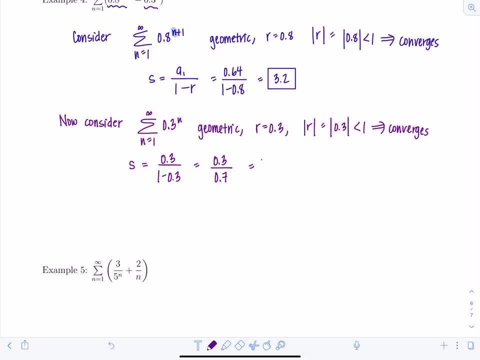 So that's 0.3 divided by 0.7, which is 3 sevenths. So what does this tell me now? Well, according to my theorem, then, the difference of these two series must also be convergent. So the sum n equals one to infinity, of 0.8 to the n, plus one minus 0.3 to the n. 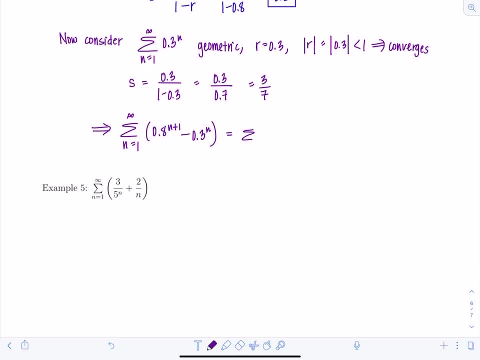 now I'm allowed to distribute the summation across: the sum n equals one to infinity of 0.8 to the n, plus one minus. the sum n equals one to infinity of 0.3 to the n. This would equal 3.2 minus 3 over 7, and then getting a common denominator, this is 97 over 35.. 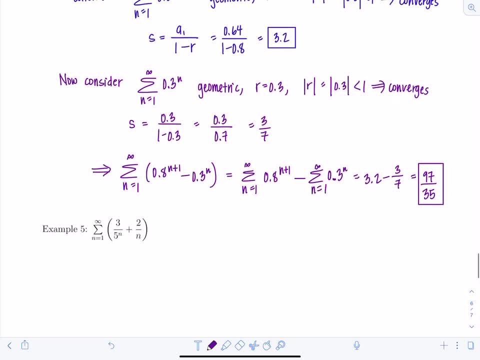 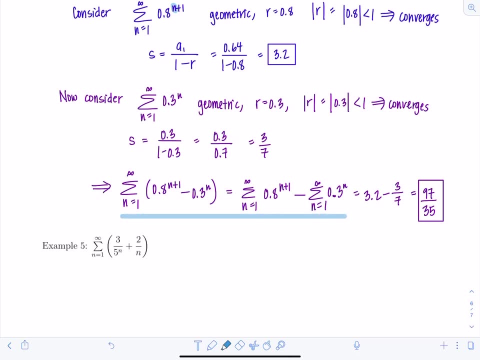 Okay, so your work needs to be done in this way. You are not allowed to distribute or write this statement until you've first shown and justified that each of these series is indeed convergent. Okay, then you're allowed to write that last line that I have. 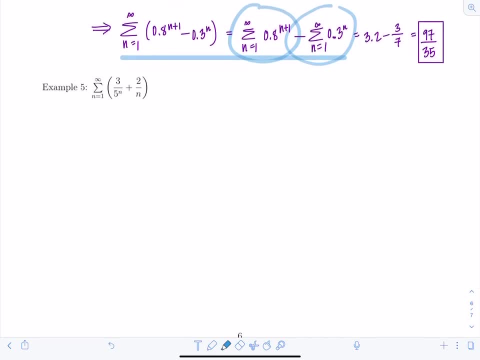 Okay, last example for the lesson. We have the sum n equals one to infinity, of three over five to the n, plus 2 over n. Okay, so first let's consider 3 over 5 to the n. So we have the sum n equals 1 to. 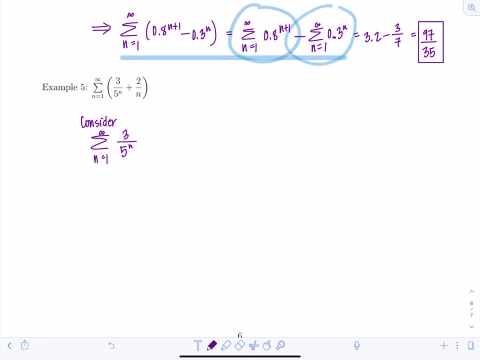 infinity of 3 over 5 to the n and I can take the 3 outside the sum. n equals 1 to infinity and I have 1 fifth to the n. Now this is geometric again, absolute value. of r is the absolute value. 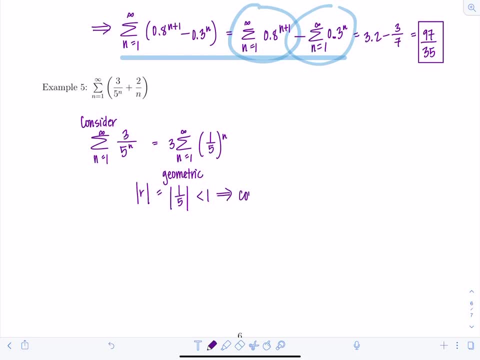 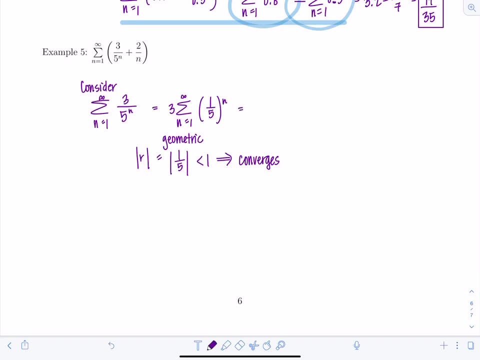 of 1 fifth, which is less than 1, and that converges So I can find its sum. This is going to be equal to 3 times a1.. So if I substitute in 1 for n, I'm going to have 1 fifth over 1 minus r. 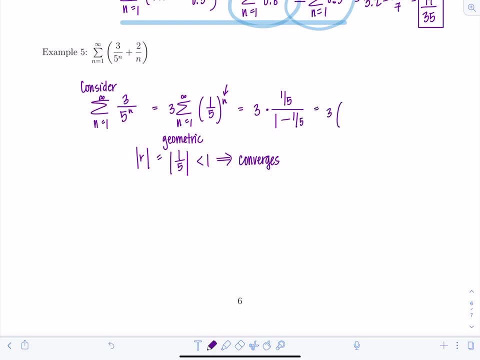 1 minus 1 fifth. So that's going to be 3 times 1. fifth. divided by that's going to be 4 over 5, or times 5 over 4, 5s are going to cancel. so this is 3 fourths. 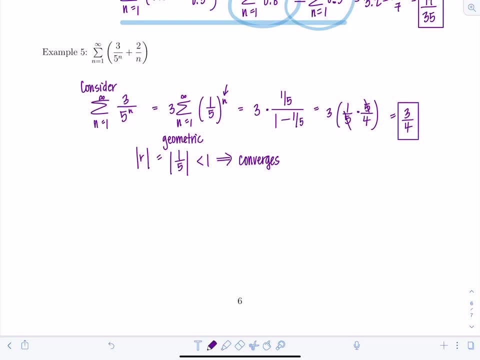 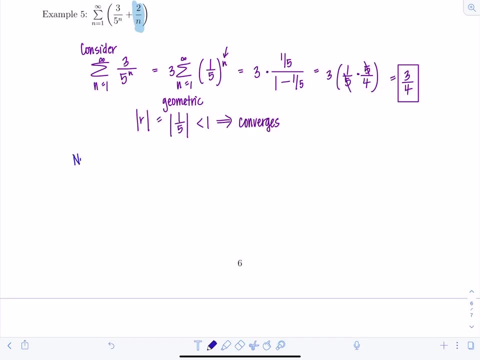 Okay, so that's the sum of that little series. Now I'm going to consider the second part: 2 over n. So now consider the sum n equals 1 to infinity of 2 over n. Well, this is 2 times the sum of n equals 1 to infinity of 1 over n, and this, I know, is the harmonic series. 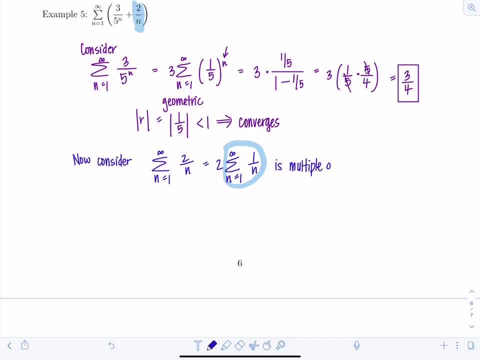 So 2 times that is a multiple of the harmonic series. and what did we just say about the harmonic series on the previous page? It actually diverges. We'll show why later. So what does that mean about my overall series? Well, if one part diverges, the whole series.